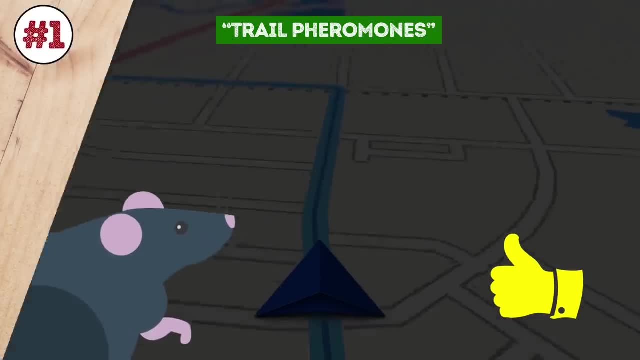 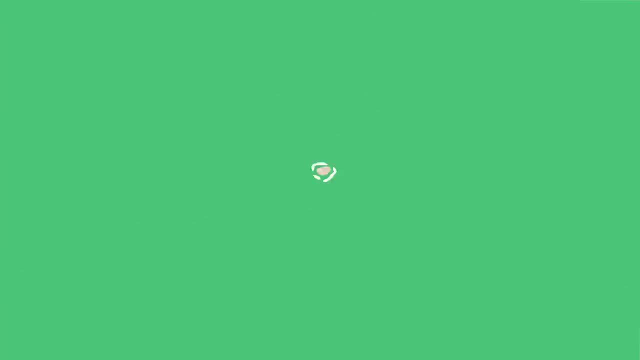 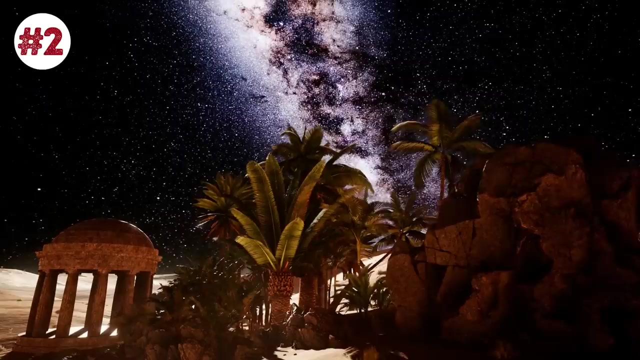 Pretty cool, huh? Not for homeowners, though. Add some peppermint oil to your cleaning solution and mop your floor with it to wipe away their little trails. Number 2. Basil. People have been using plants and herbs to keep pests at bay, probably since the dawn of time. Our ancient ancestors were the first to boil, stew, burn and crush leaves to make natural bug repellents. A prime example is basil. Studies published in 2009 in the Tanzania Journal of Health Research and the Journal of Cellular Biology found that lemon basil and cinnamon basil could effectively repel the Anopheles gambiae complex. 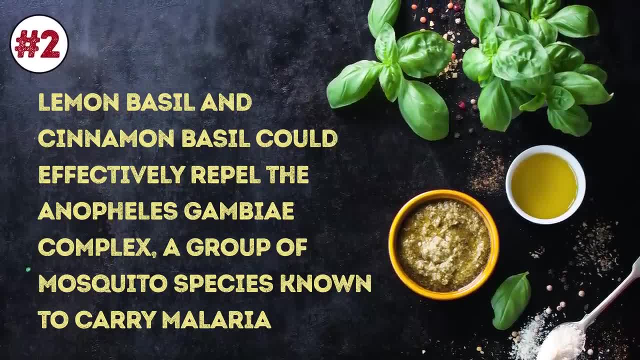 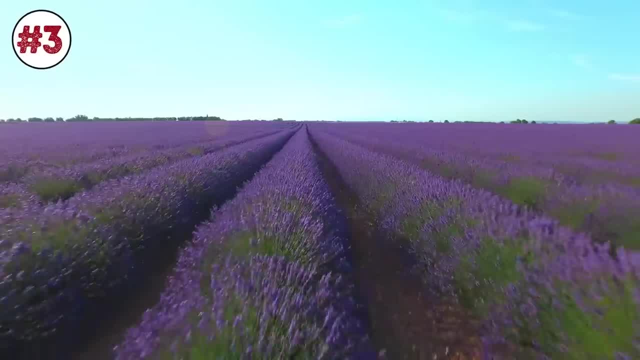 a group of mosquito species known to carry malaria, Number 3. Lavender: Its soothing fragrance relieves us from stress and calms our nerves. It does quite the opposite for mosquitoes, houseflies, fleas and moths, though. Lavender scent can protect us from diseases, diseases and diseases. Lavender scent can protect your home, pets and other plants from being infested by bugs. You can also put lavender oil on your wrists and neck to shield yourself from mosquitoes. 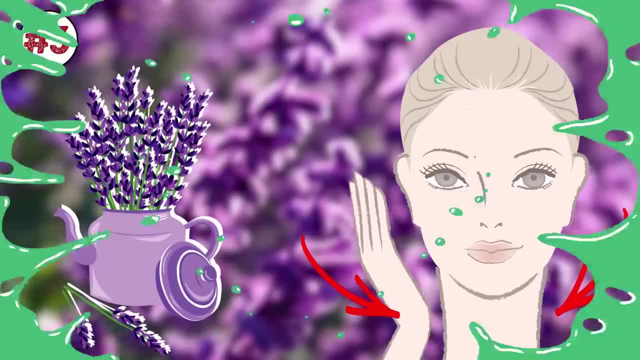 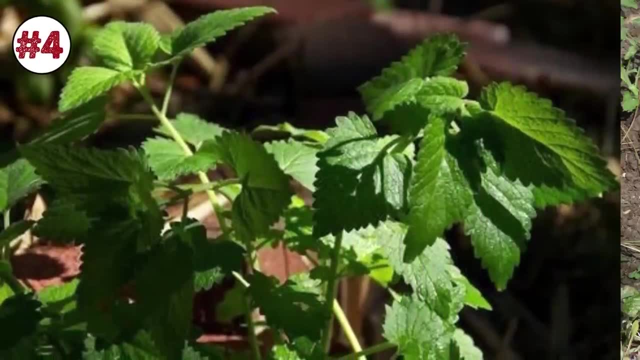 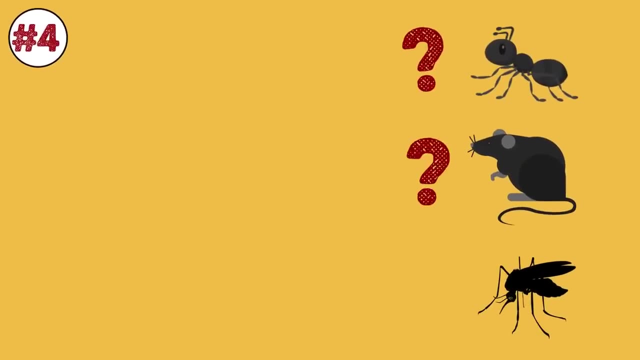 Plus, it's like an instant perfume, Number 4. Catnip: Plant some catnip in your backyard, and your furry feline companion will greatly appreciate it. As for ants, mice and mosquitoes, Eh, not so much, According to research. 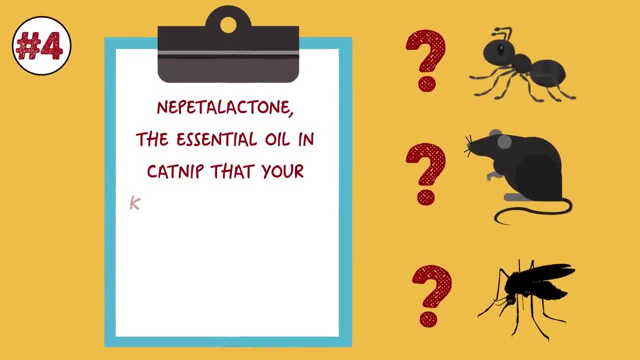 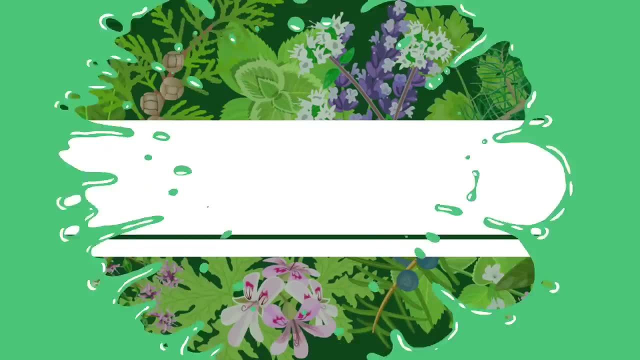 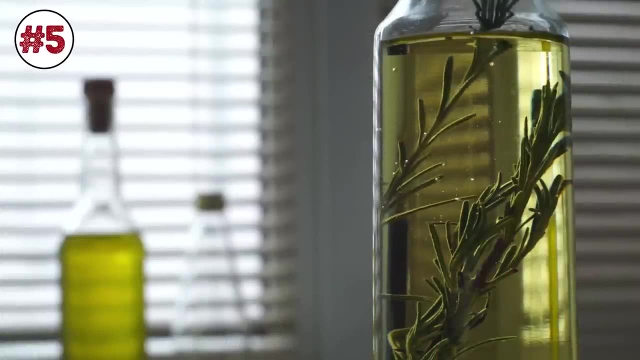 Nepetalactone, the essential oil in catnip that your kitty loves so much, acts as an irritant against these common household pests. Number 5. Rosemary: This needle-like herb is commonly used in cooking and has medicinal properties. It also attracts butterflies, but deters flies and mosquitoes. 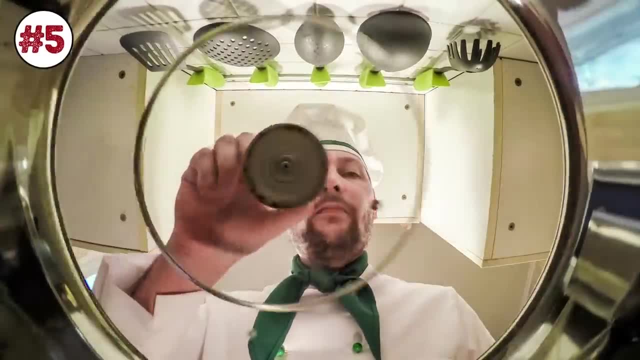 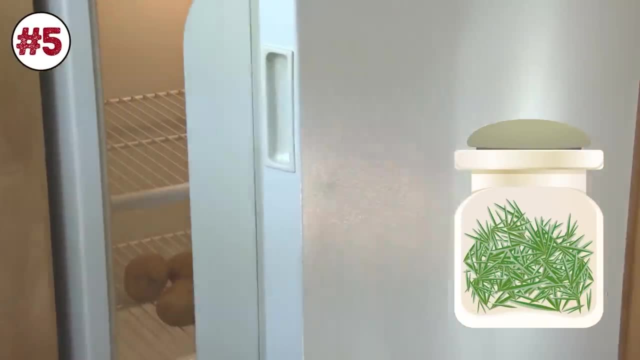 Make a non-toxic bug spray out of it by boiling some dried rosemary leaves in water, Then mix in some cool water and put it in a container, Store the rosemary water in the fridge and later pour it into some spray bottles. 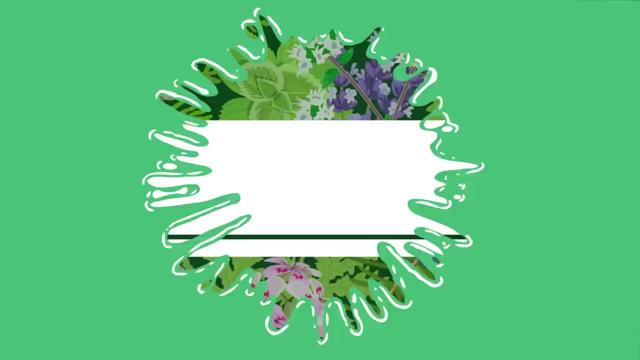 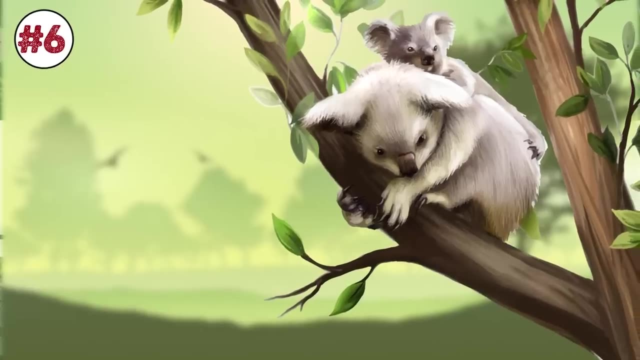 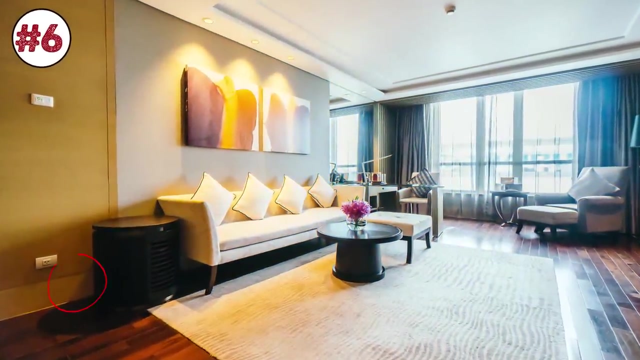 Easy peasy. Number 6. Eucalyptus essential oil. Koalas can't live without this plant. Spiders, however, will stay far away from it at all costs. Apply a few drops of eucalyptus essential oil to some cotton balls. 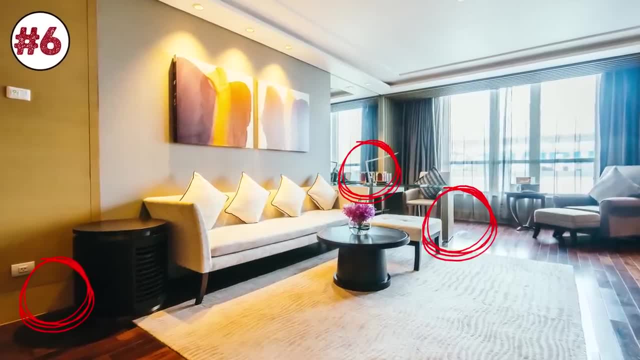 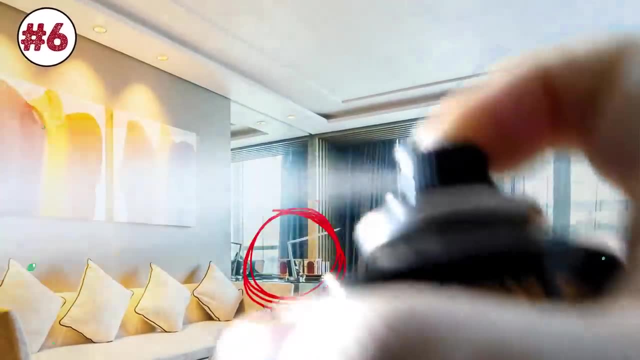 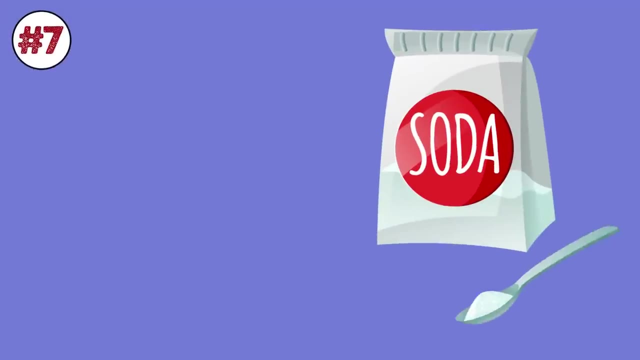 and put them in areas where you often find these eight-legged creepy crawlies. Pour it in a spray bottle to drench hard-to-reach areas like ceilings and behind large pieces of furniture. Number 7. Baking soda- Ah, the famous sodium bicarbonate. 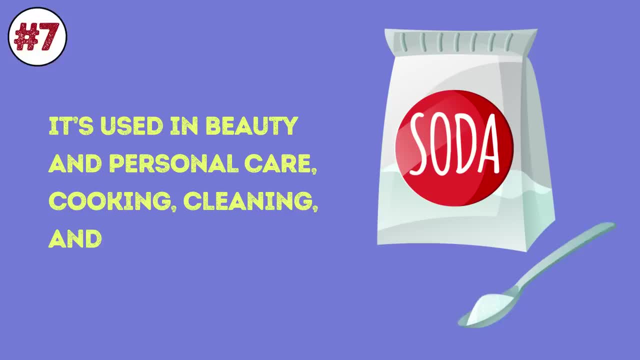 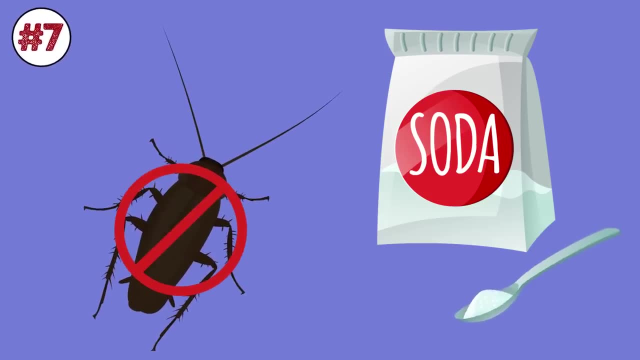 It's used in beauty and personal care, cooking, cleaning and deodorizing your house, just to name a few. You can go ahead and add insect repellent to the mile-long list of ways to use baking soda. Mix baking soda with sugar. 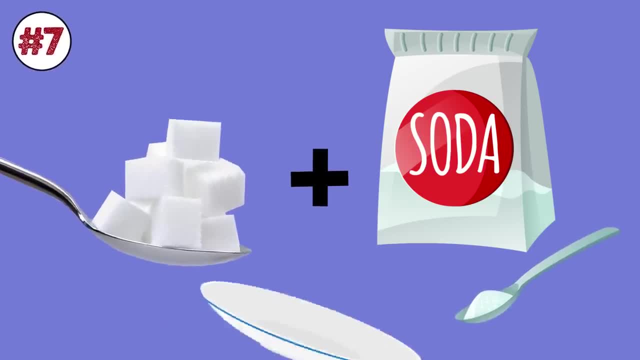 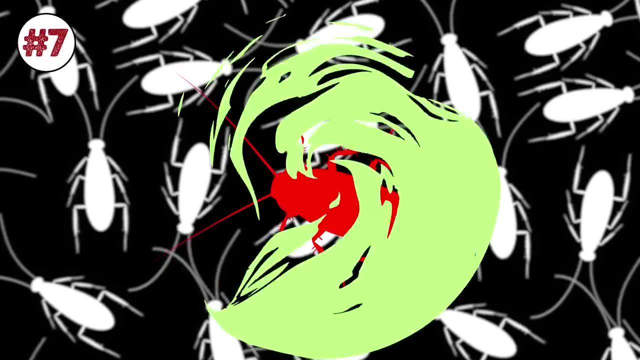 the sweet stuff will act as a bait for roaches and place a bowl of water near it. This lethal trio creates a chemical reaction inside the roach's stomach which, let's just say, won't end well for the little buggers. 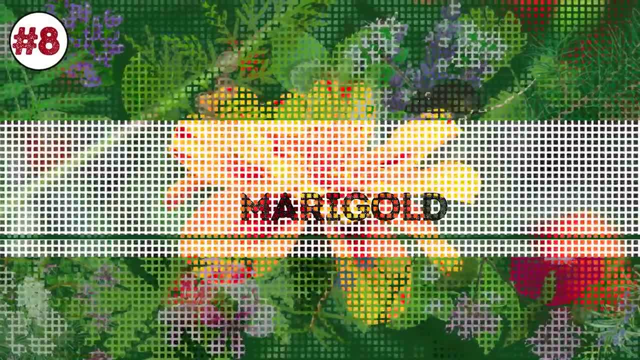 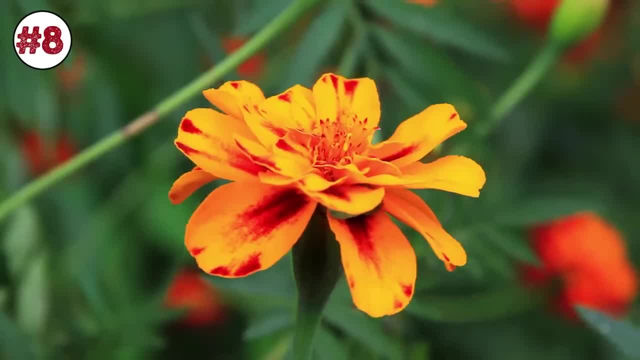 Number 8. Marigold, This ornamental plant in the daisy family, looks so innocent at first glance, Yet this beautiful, bright-colored flower can repel all kinds of pests like mosquitoes and flies. Marigold contains pyrethrum. 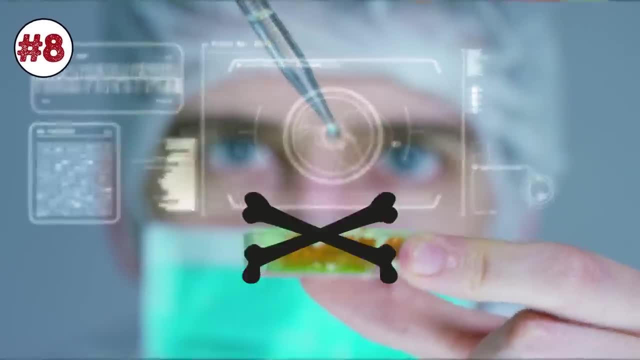 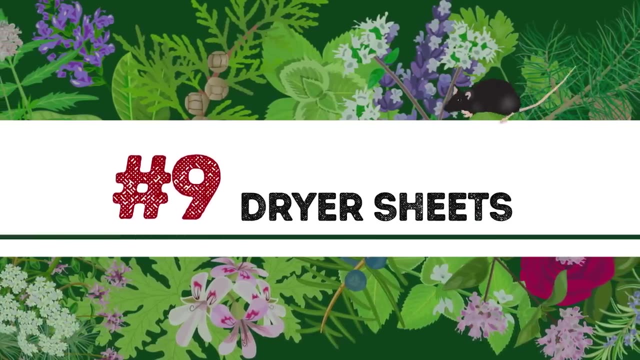 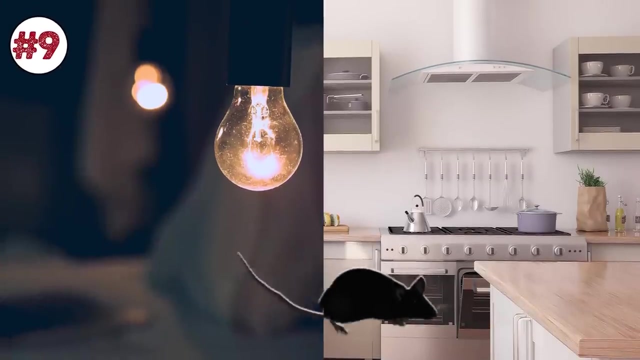 a compound that's commonly found in commercial bug sprays. Pretty but lethal Yikes, Number 9. Dryer sheets. The favorite hangout spots for mice are the kitchen attic, inside the walls under the floorboards and any other dark, secluded areas. 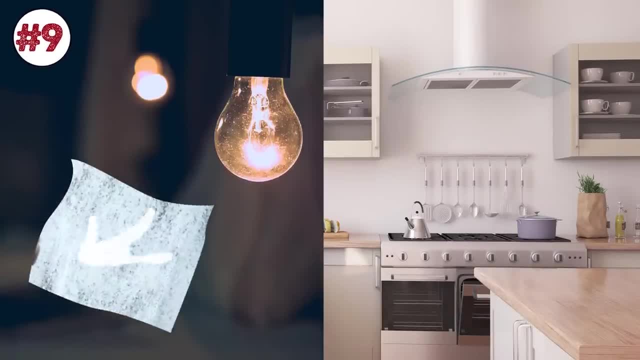 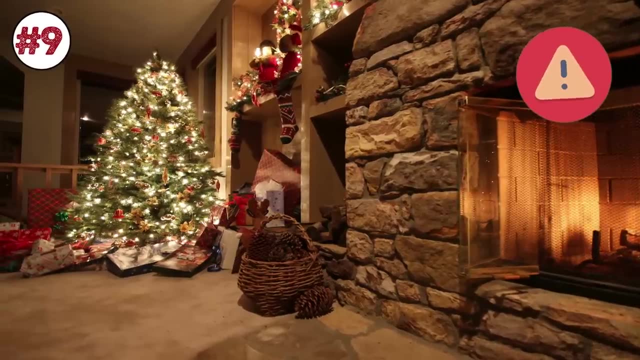 Hey, they have standards too, you know. Put original scented dryer sheets in these places to keep mice out. Just remember that this technique is only a preventative measure and probably shouldn't be used if mice have already set up camp inside your home. 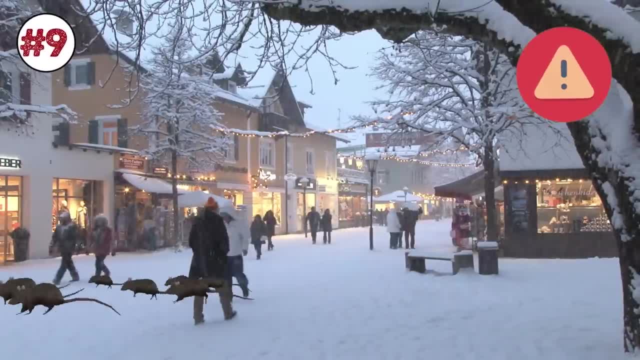 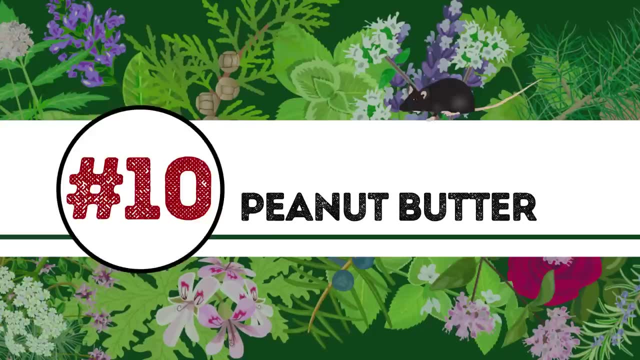 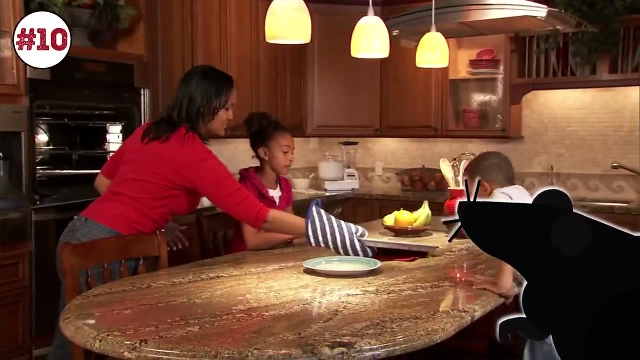 You don't want them scurrying out in the open because they have no place to go, do you, Number 10.. Peanut butter Mice and rats love to help themselves to our kitchen cabinets, food pantries and anywhere else they can stuff their bellies full at our expense. 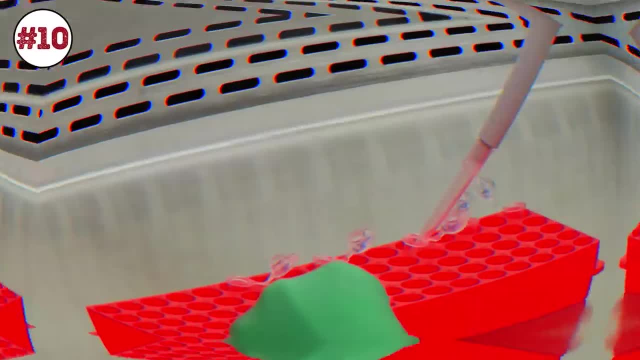 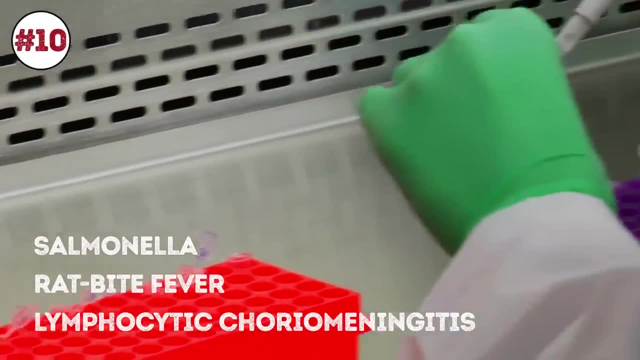 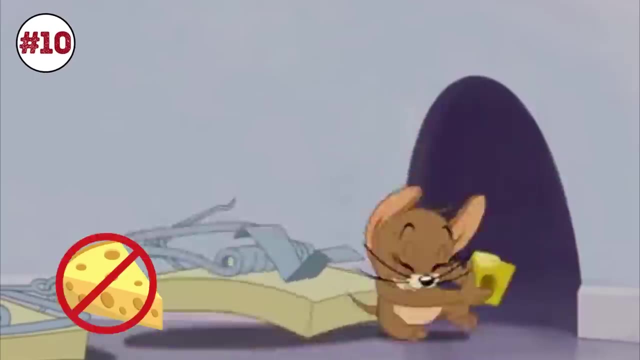 And how do they show appreciation? Well, according to the Centers for Disease Control and Prevention, rodents can infect people with salmonella, rat bite fever and lymphocytic choriomeningitis. Protect yourself and your family by setting traps with no nut cheese. 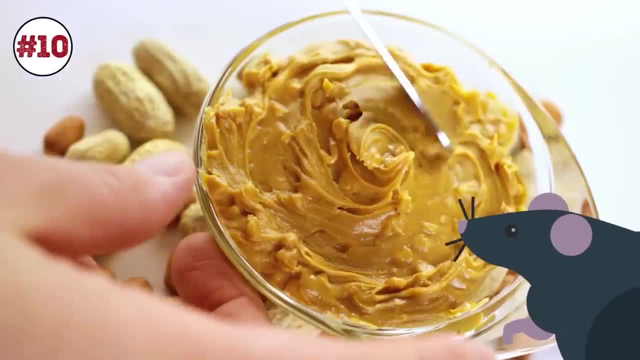 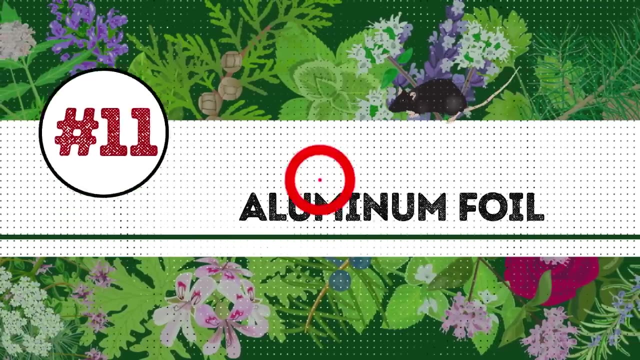 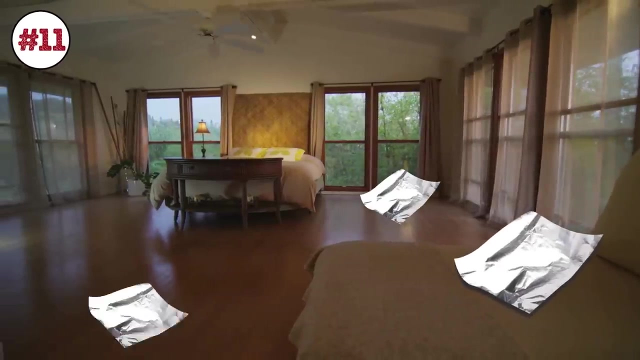 peanut butter. Mice can't resist this delicious yet deadly treat. Number 11. Aluminum foil. Mice are highly sensitive to sounds, especially metallic sounds. Mouse-proof your house by placing sheets of aluminum foil in their hideouts. They'll avoid those spots in the future. 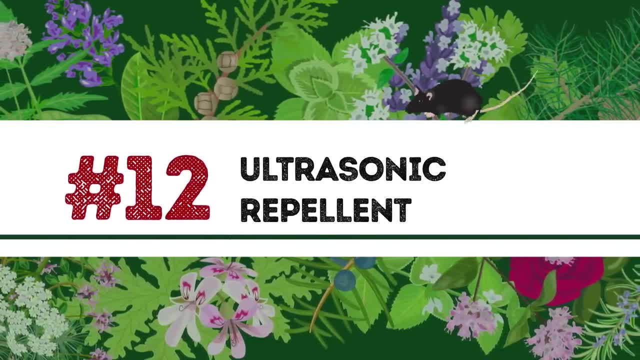 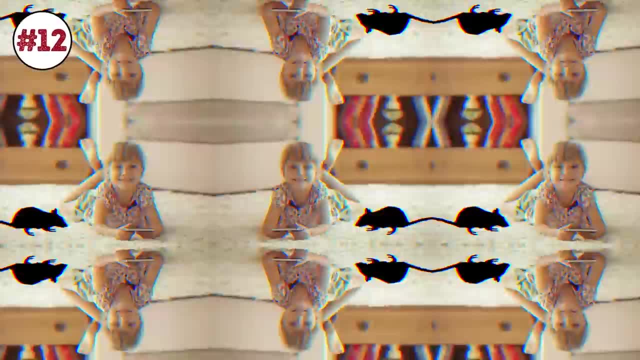 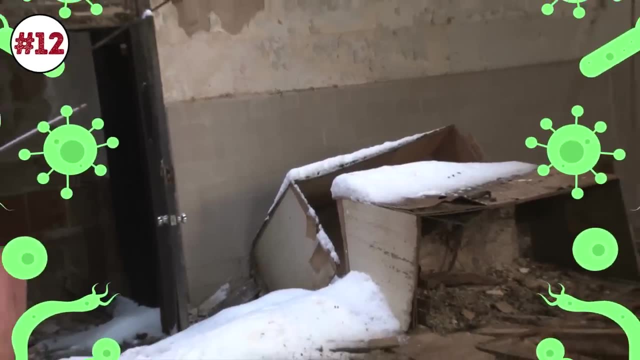 Number 12.. Ultrasonic repellent Mice aren't just known to carry diseases. Another reason why they're called pests is that they wreak havoc on your house. They chew the beams inside the walls and tear holes in the drywall. Oh, and let's not forget about all those bacteria-filled droppings. they sprinkle throughout your home- Just lovely. If, at this point, you've tried just about everything, from traps to getting a cat and nothing seems to work, or you're allergic to cats, or whatever the case might be, you can always try ultrasonic repellents if you're willing to spend the money. 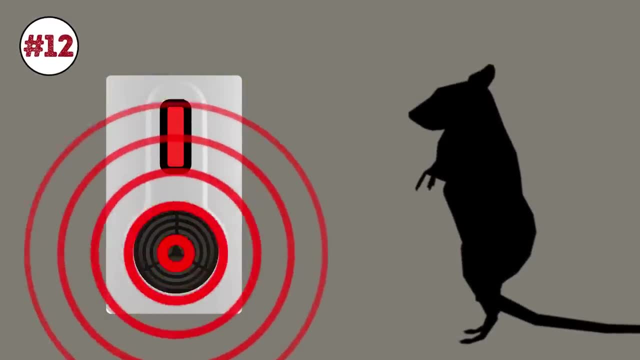 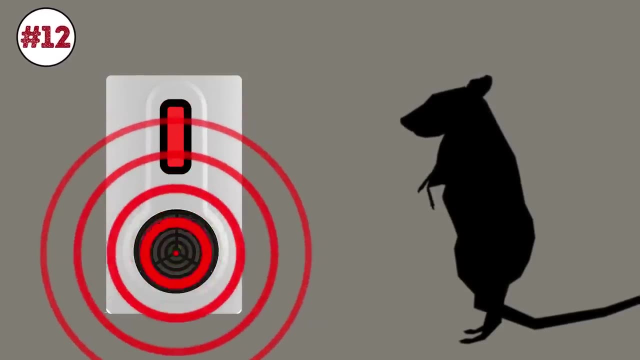 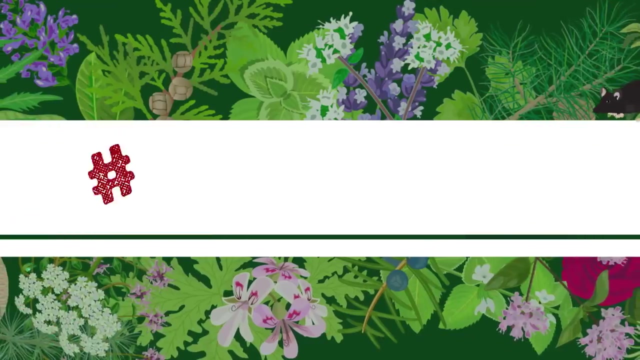 These things emit high-frequency sounds that are only sensitive to a mouse's ears. However, skeptics claim that this sophisticated device doesn't work and lacks scientific backing. So use this type of repellent at your own risk. Number 13. Borax. 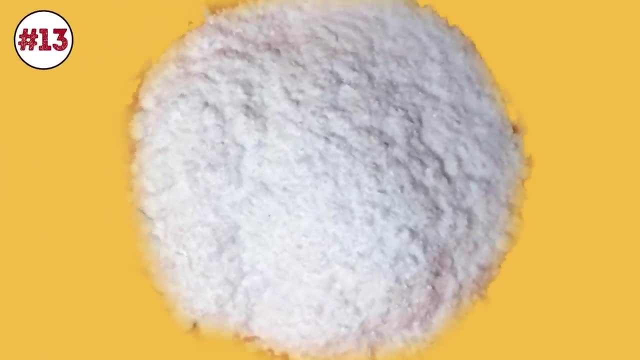 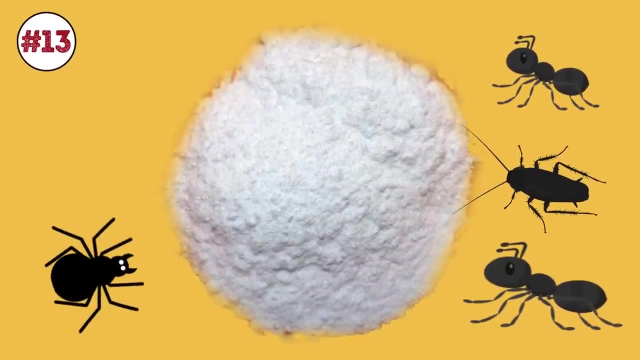 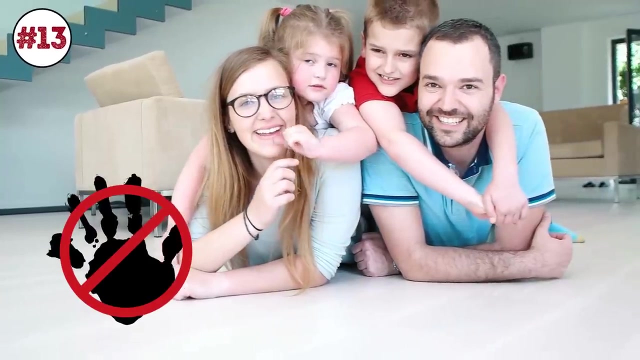 This white crystalline compound is used as a cleansing agent and in glassmaking. It can also kill ants, roaches, termites, spiders and even mold. To make sure your target will approach it, use honey or sugar as bait. As a safety precaution, make sure your borax concoction is far out of reach of children. 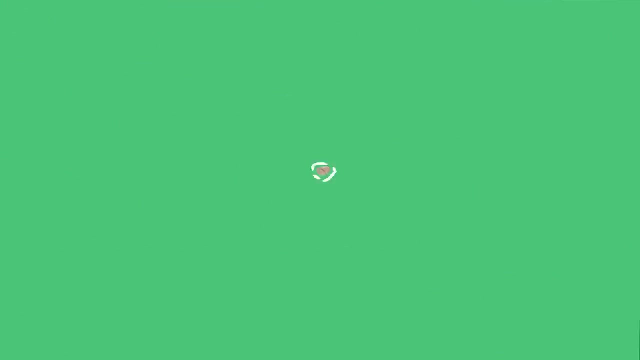 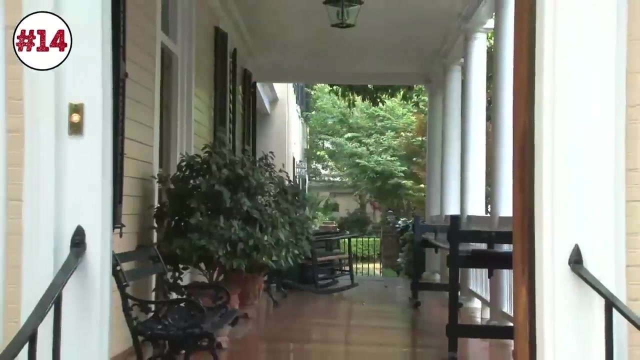 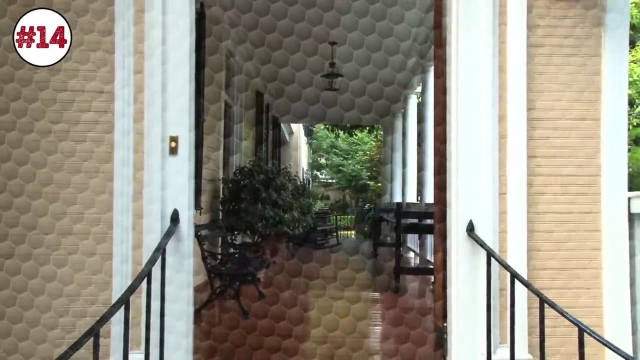 Also wear a face mask and gloves when using it. Number 14. Steel wool or copper mesh. They say prevention is the best cure, So seal any possible entryways, even the tiniest little cracks, so that mice can't even get into your home. 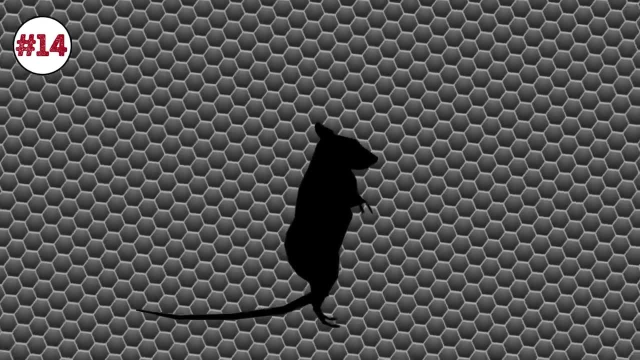 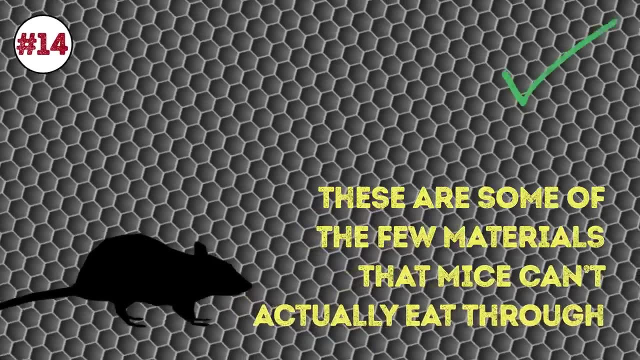 To do this, use steel, wool or copper mesh to mouse-proof your house and seal the deal with caulking. These are some of the few materials that mice can't actually eat through, so they're great at keeping rodents out. Number 15. Cayenne pepper. 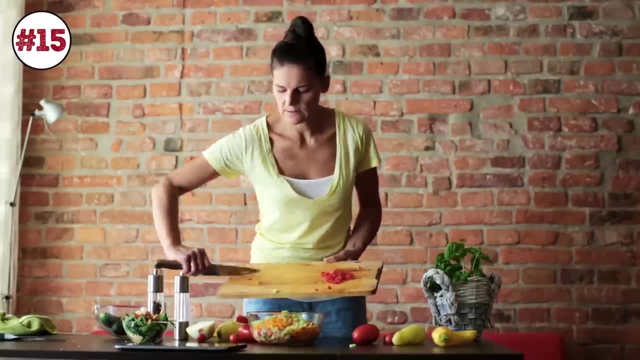 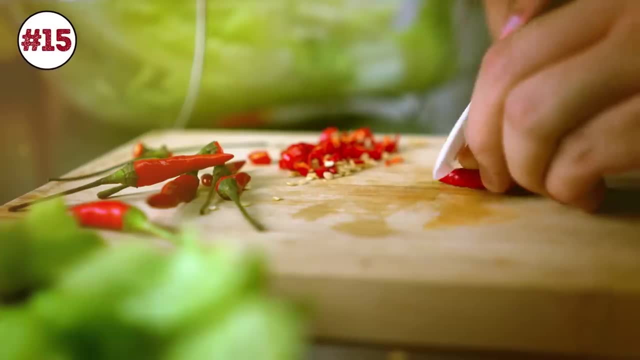 Yet another tasty ingredient used in cooking that can also keep pests away from your personal space. If you need to keep wild animals out of your garden, cayenne pepper is a perfectly safe way to keep them at bay. Just sprinkle it on the topsoil to keep rabbits and squirrels. 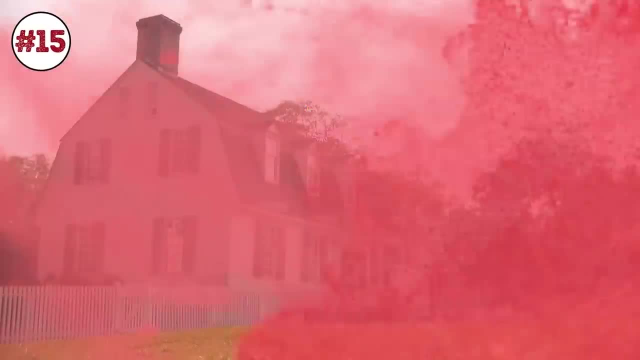 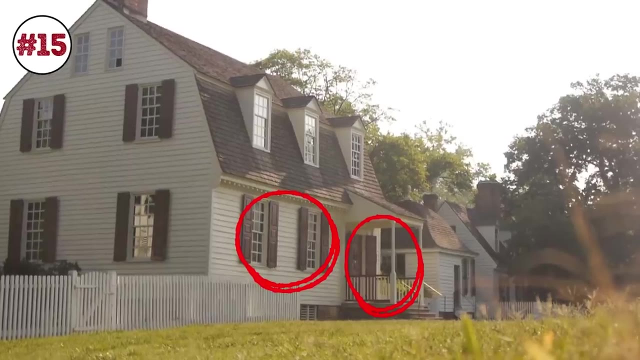 from munching on your fresh veggies. You can also sprinkle cayenne pepper around your home, especially near entry points like doors and windows, to keep ants, roaches and other creepy crawlies from invading your home Number 16.. Neem.